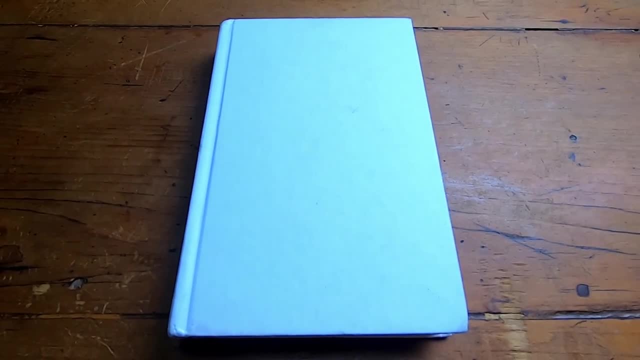 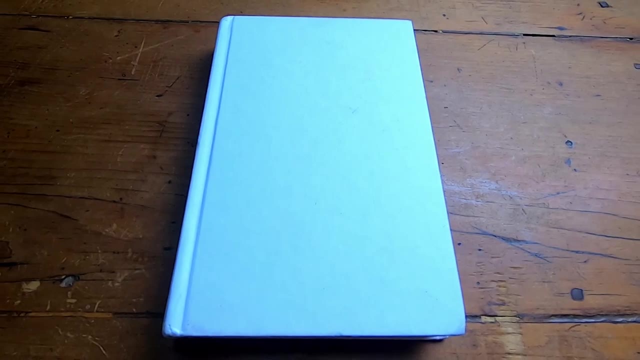 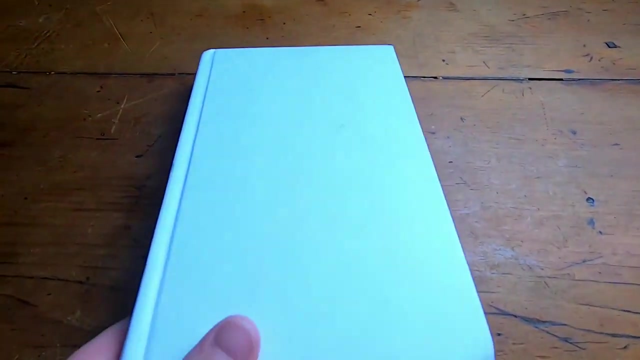 Hi everyone. In this video I want to talk about what I think is possibly the absolute best book for anyone who wants to start with calculus, And there are several reasons why I think this is the best book. Before I talk about that, let me just show you what book this is. It's kind of different. It's got a white cover. 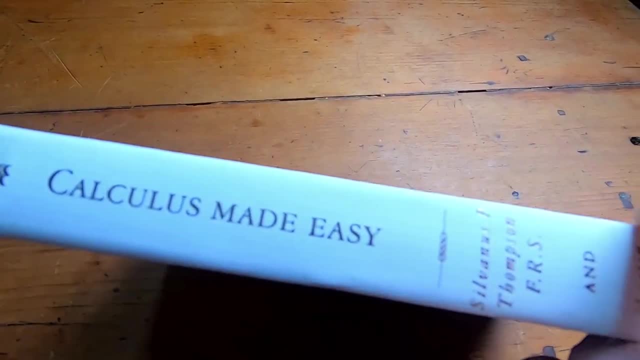 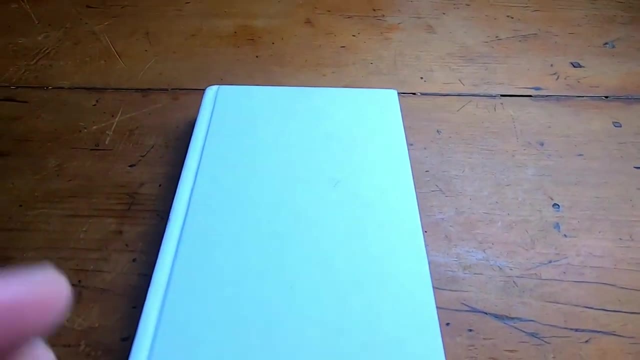 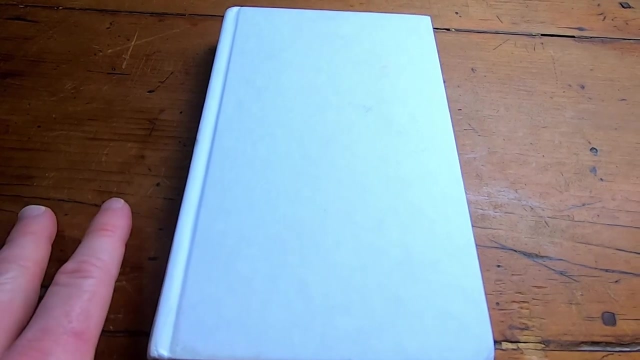 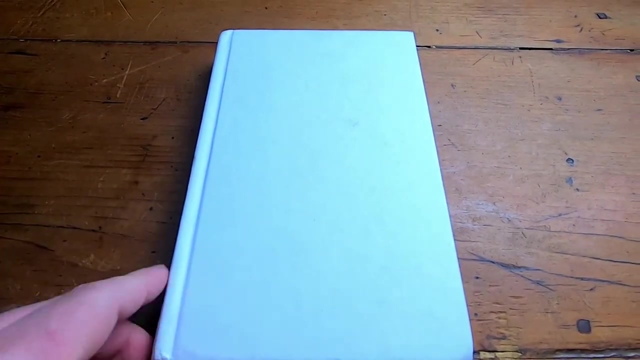 and the book is Calculus Made Easy by Sylvanus Thompson and Martin Gardner. This book is absolutely incredible. I believe this book was first published in 1910.. Sylvanus Thompson was actually a physicist and I believe he was also an electrical engineer And he published many books on engineering and math and I 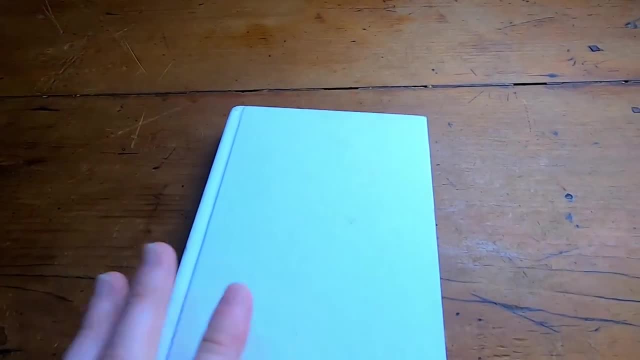 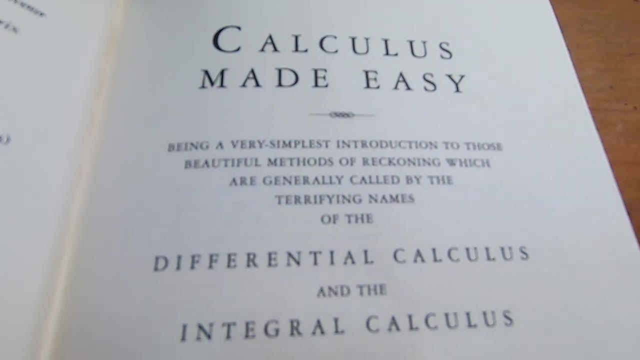 think this might be his most famous work. Let's take a look inside this amazing book and talk about why. This is the inside of the cover. This is just awesome: Calculus Made Easy, Being a very simplest introduction to those beautiful methods of reckoning which. 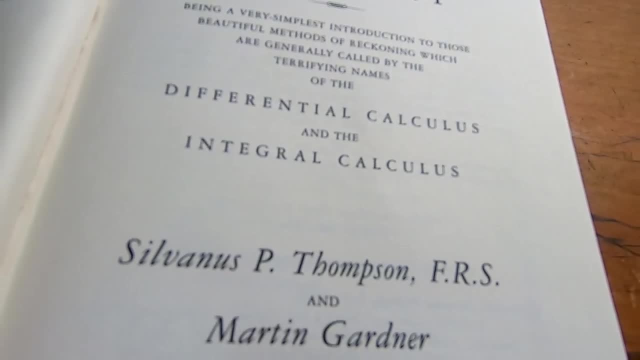 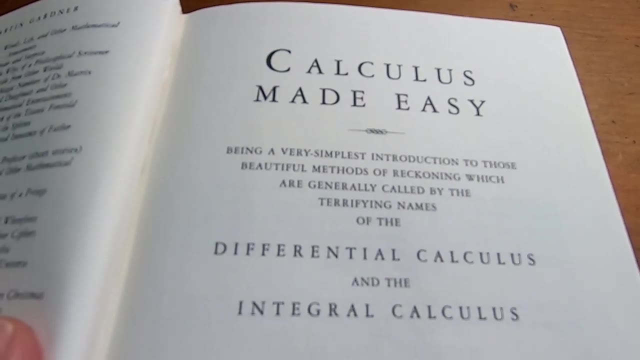 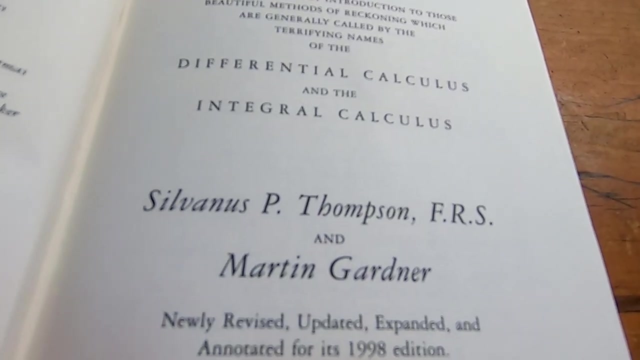 are generally called by the terrifying names of the differential calculus and the integral calculus. So he was kind of a game changer right, Trying to write a book in a very understandable way during an era of rigor and formalism. And he was no fool. Sylvanus Thompson was a pro, A very, very smart man. This book contains: 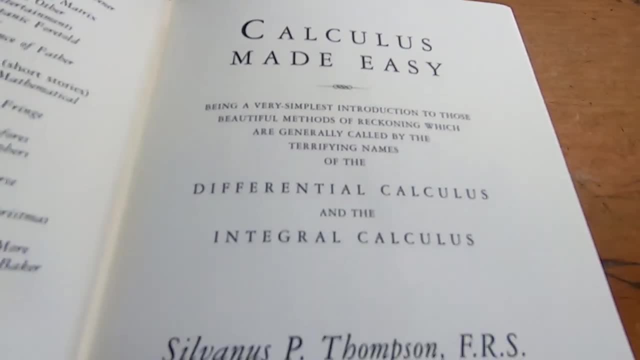 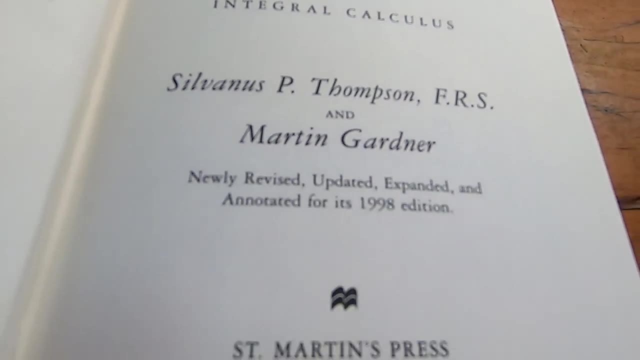 very correct methods of reckoning And he wrote a book called Calculus Made Easy. It's called Correct Mathematics, so don't let the title fool you. This is newly revised and updated and expanded and annotated for its 1998 edition. Here we go. The original edition of Calculus Made Easy was written by: 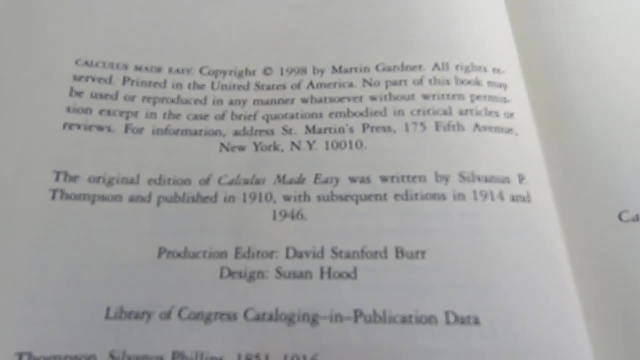 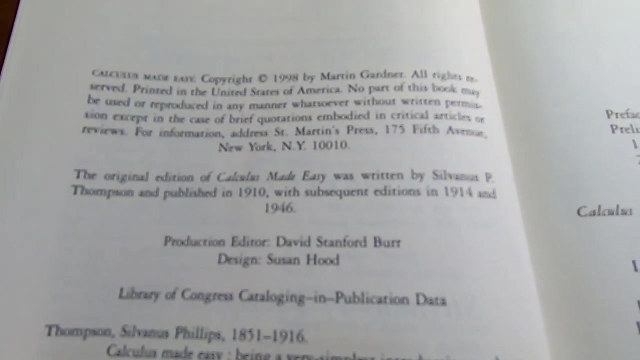 Thompson and published in 1910, with subsequent additions in 1914 and 1946.. This book has survived the test of time, and for a reason. I really think Sylvanus Thompson was a genius in his own working on Calculus Made Easy. But for a reason I really think Sylvanus Thompson was a genius in his own work. 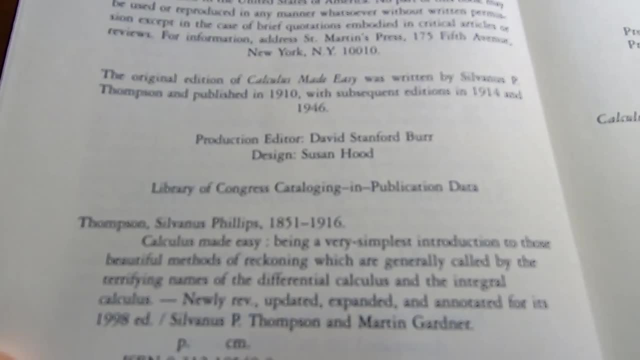 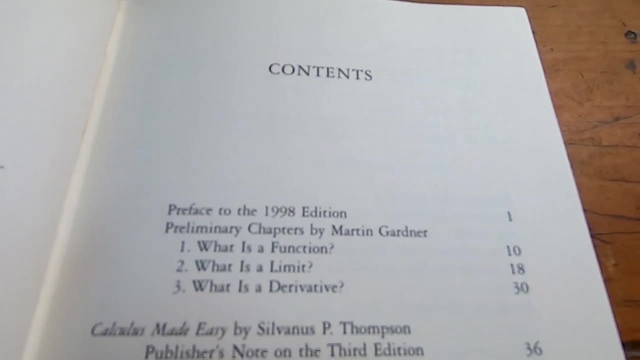 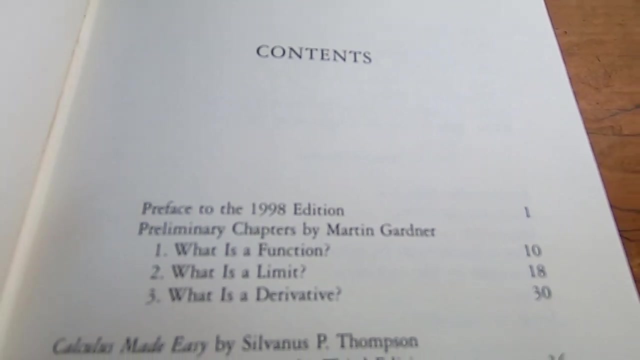 own way. I mean to be able to write a book. this good is just absolutely amazing. Even the table of contents is interesting. It's hard to find a book where the table of contents is like: whoa, this is really cool. So there are some preliminary chapters by Martin Gardner, which are awesome. 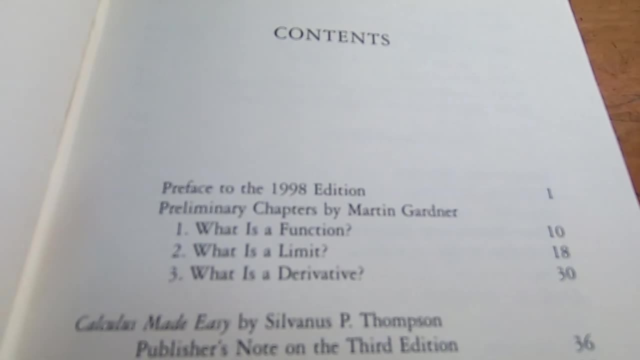 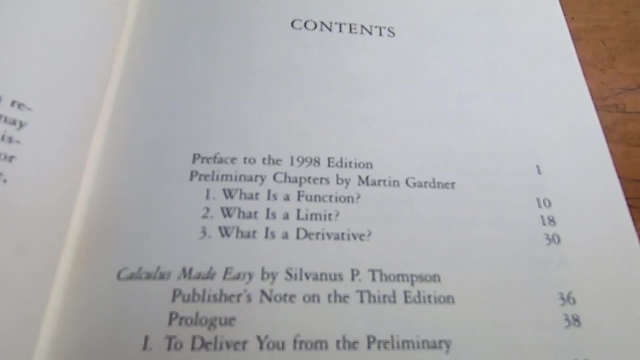 Starts off by talking about what a function is, what is a limit, what is a derivative. And I have read all of these chapters, the preliminary ones so far, And then we have the contents. I'm just going to go slowly so you can see, So to deliver you from the preliminary. 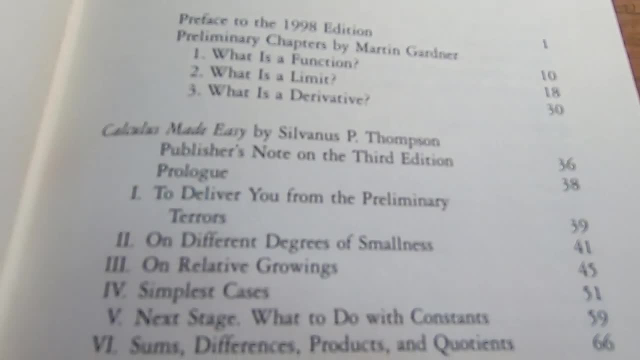 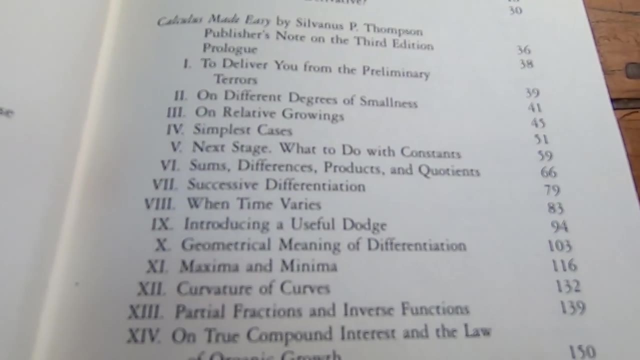 terrors. This is a calculus book and it's not, like you know, calculus for dummies. I know the name makes you think that it's not like a real calculus book. It is, and the author was a very, very pro-mathematician. 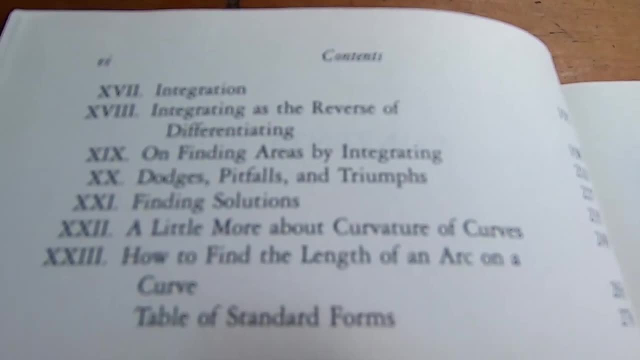 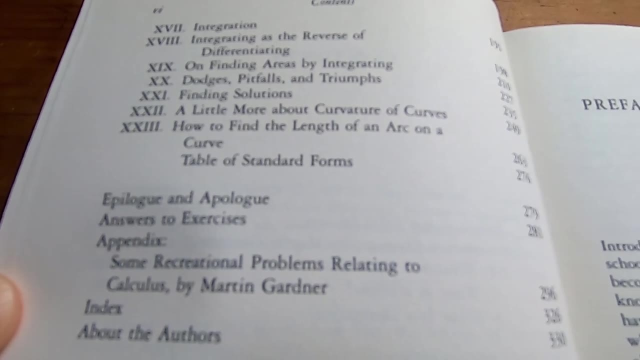 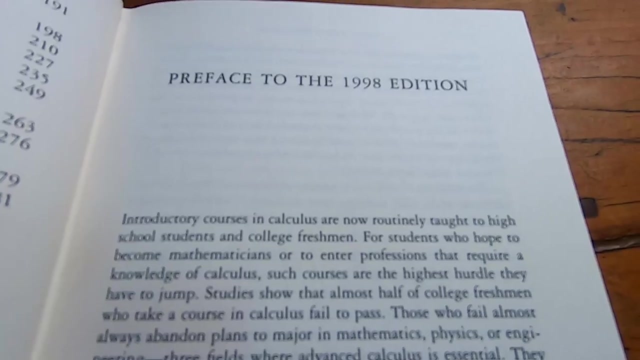 And here is the rest of the table of contents, And it includes answers to every single exercise. Every single exercise has a solution in the back of the book. I mean, that has to be like unheard of for a book published so long ago. Even the preface is good. Let's go ahead and read it together or part of. 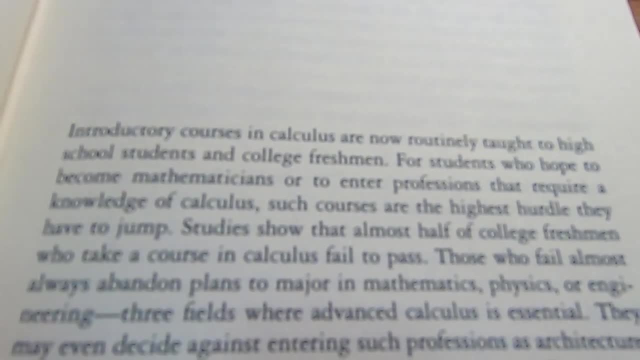 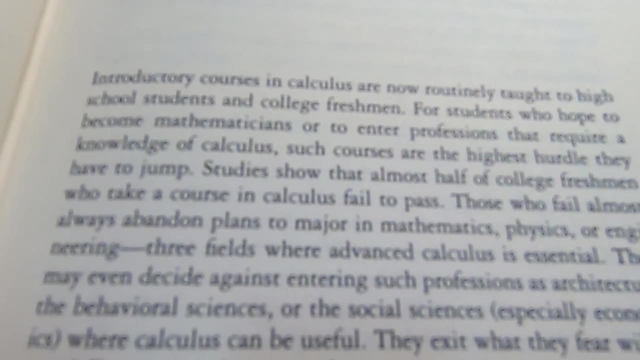 it. Introductory courses in calculus are now routinely taught to high school students and college freshmen. For students who hope to become mathematicians or to enter professions that require knowledge of calculus, such courses are the highest hurdle they have to jump. This is true. 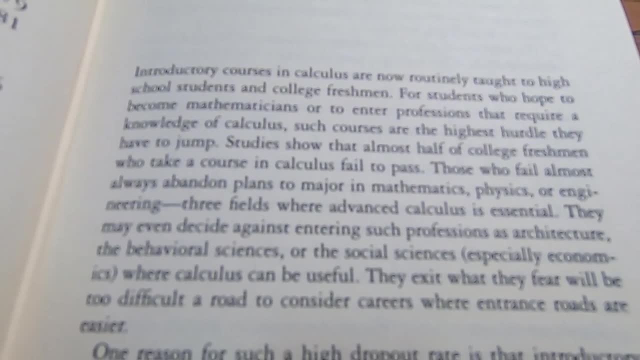 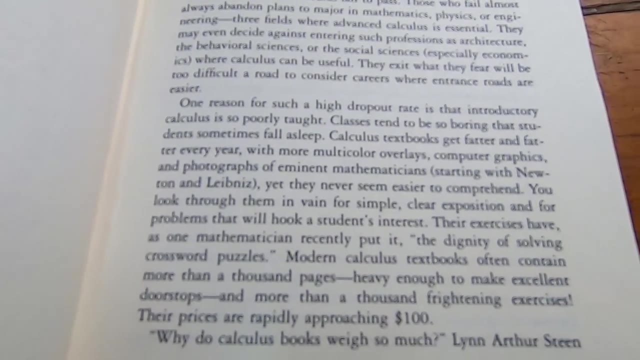 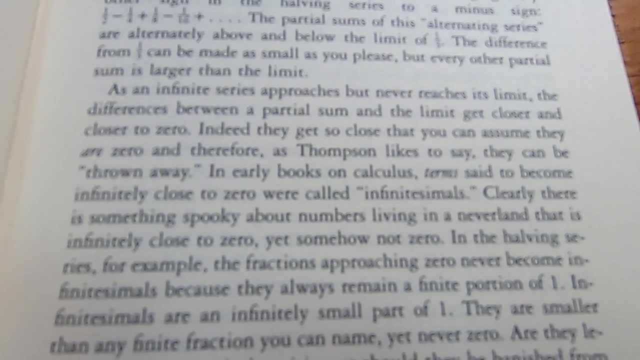 Studies show that almost half of college freshmen who take a course in calculus fail to pass, And it goes on and on and on. So really, really nice preface. It's worth reading. It's very, very enlightening. This is a little piece from one of the preliminary sections by Martin Gardner. 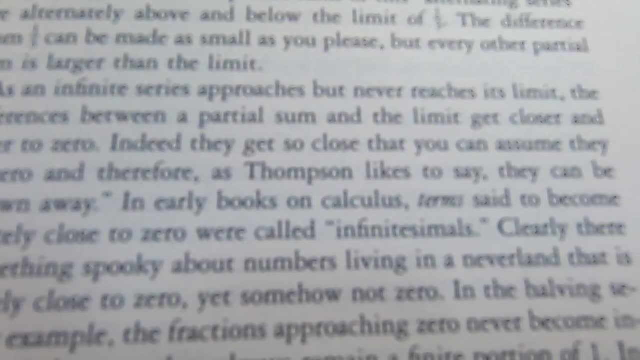 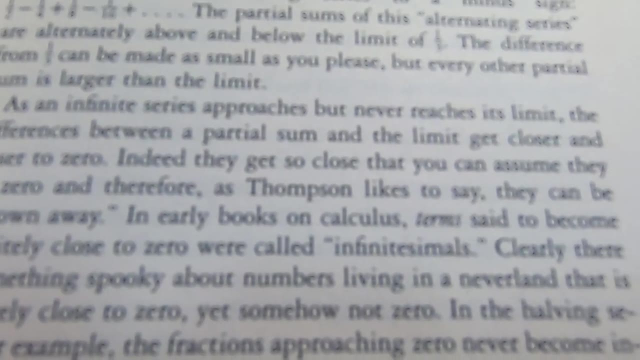 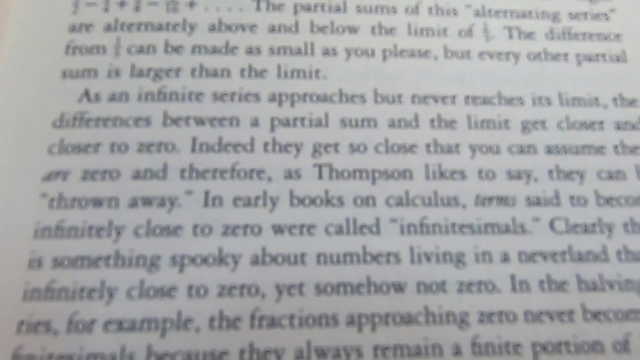 It says, As an infinite series approaches but never reaches its limit, the differences between a partial sum and the limit get closer and closer to zero. Indeed, they get so close that you can assume they are zero And therefore, as Thompson likes to say, they can be thrown away In early books on calculus. 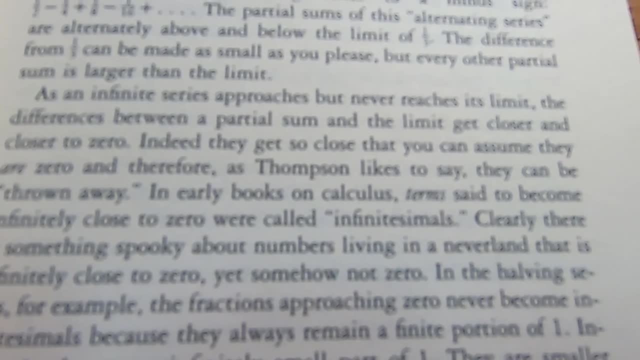 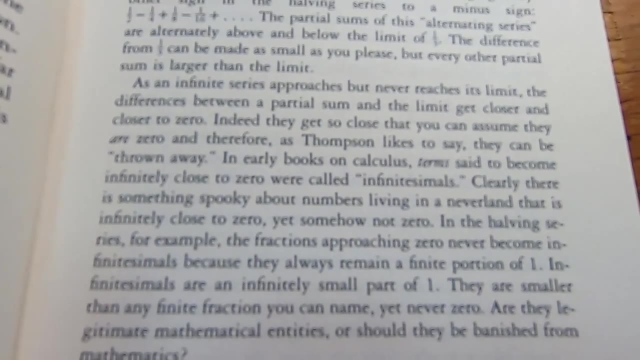 terms said to become infinitely close to zero were called infinitesimals. So Thompson uses this type of explanation throughout the book And it's really quite elegant. You can sit back and you can actually lay in bed and you can read this book. You can't say that. 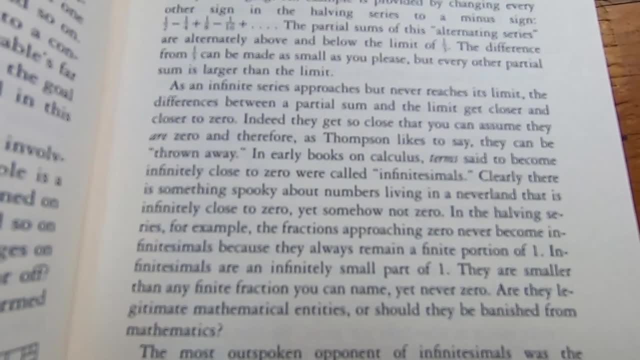 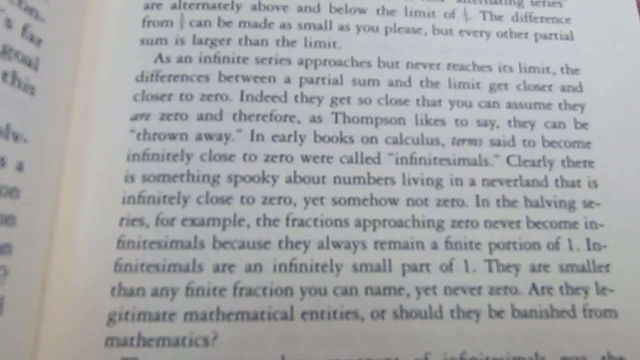 about a lot of modern calculus books. Not just that: you can understand most of it, So it's an understandable, readable calculus book which makes it perfect for beginners. He even tells you how to read derivatives. I love this. This is such an amazing book. 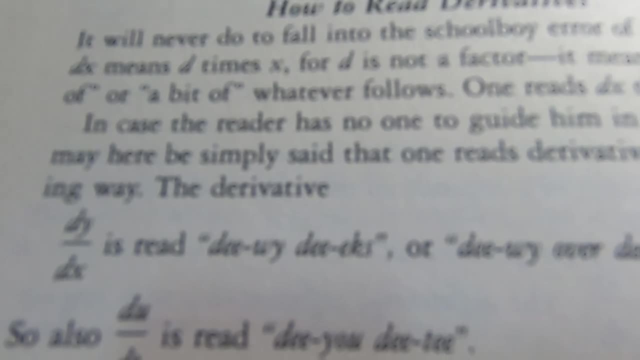 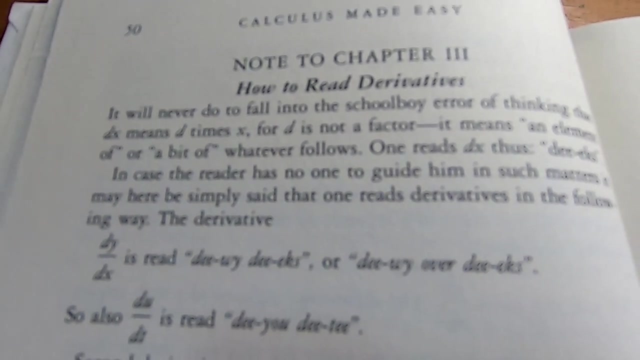 He says D-Y-D-X is read and look at that: D-Y-D-X or D-Y over D-X. I mean the effort that this man took to write this book is absolutely amazing, Admirable. I mean, there is nothing like it. There is no other book. 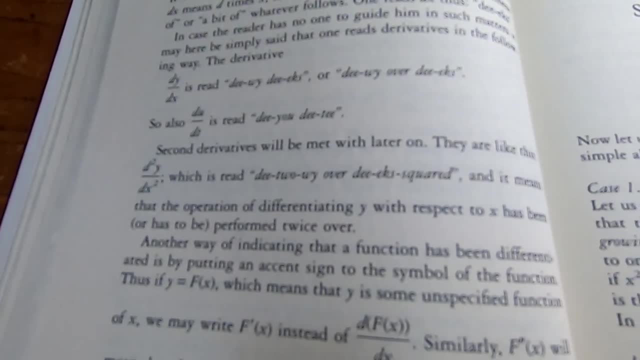 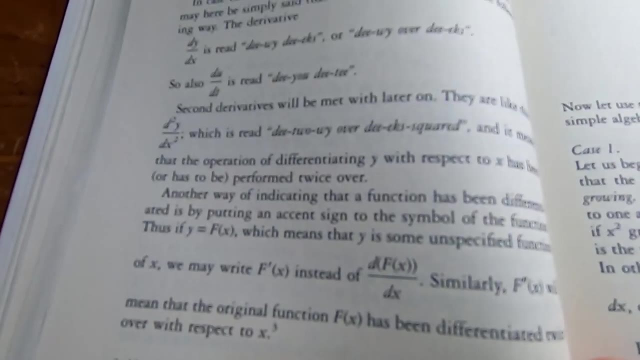 in existence on calculus that is written in this way, And I feel like to someone who doesn't know about the book or who doesn't know who the author of this book is, the name Calculus Made Easy kind of makes it lose some credibility. But don't let the name fool you. This is 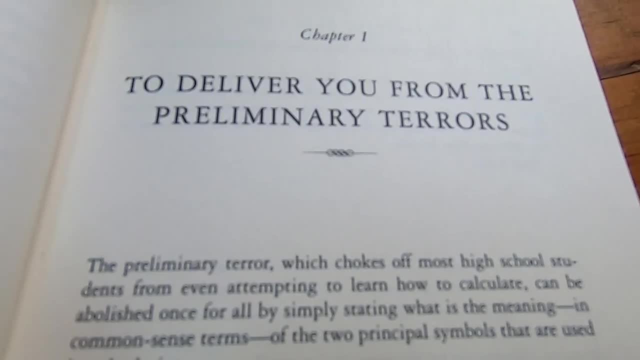 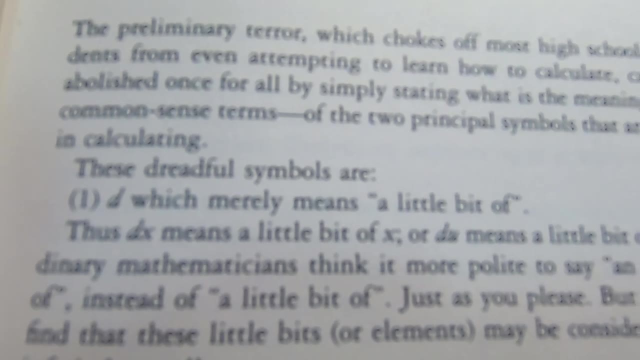 a legitimate calculus book Here. he talks about the preliminary terrors. He talks about the dreadful symptoms of calculus. He talks about the dreadful symptoms of calculus. He talks about the severeехîtettechcom, les trenacles, which merely means A little bit of. 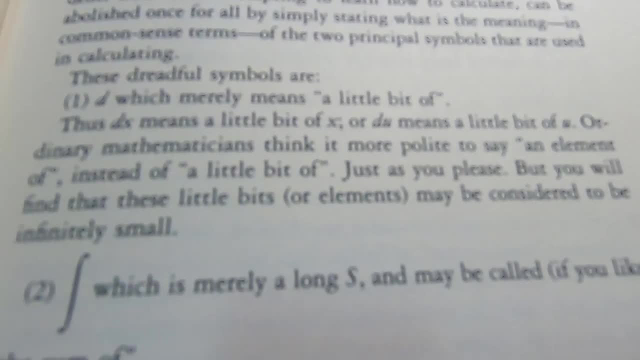 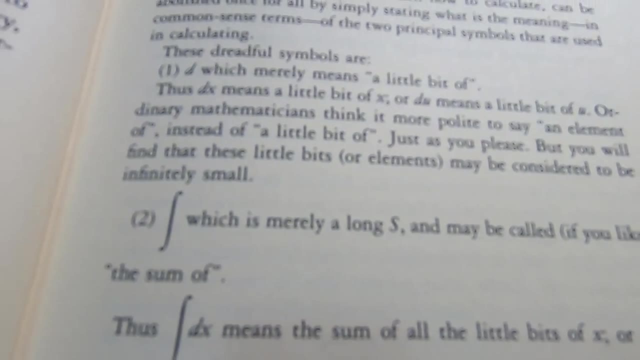 Thus D-X means A little bit of X or D-U means a little bit of U. Ordinary mathematicians think of it more politely. To say an element of, instead of saying is a little bit of, Just as you please, but you will find that these little bits or elements may be considered to be infinitely small. 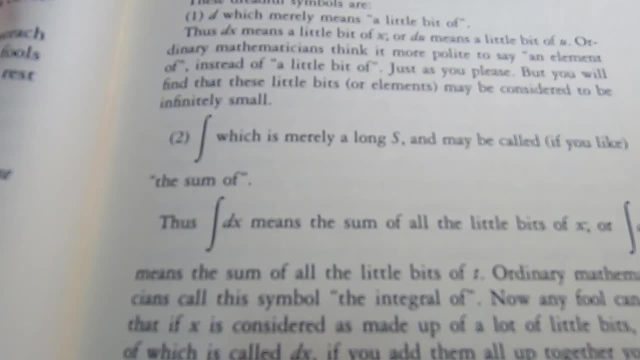 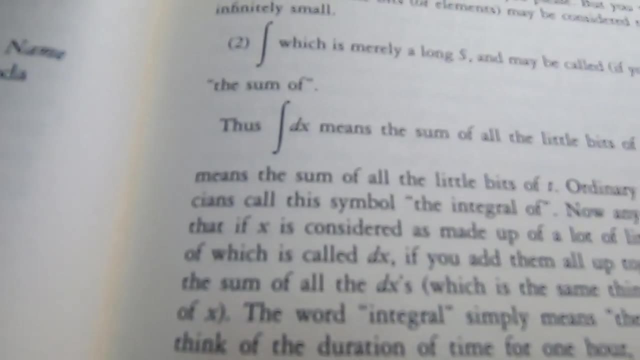 Then he talks about the integration symbol. He says its merely a long S, which it is and may be called, if you like, The sum of. I like how he says that, If you like. thus, the integral of dx means the sum of all the little bits of x, or that one means the sum of all. 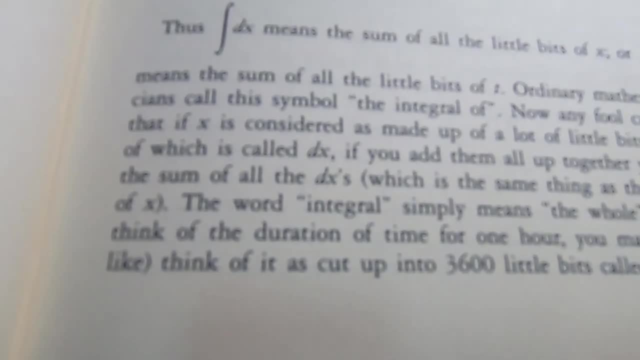 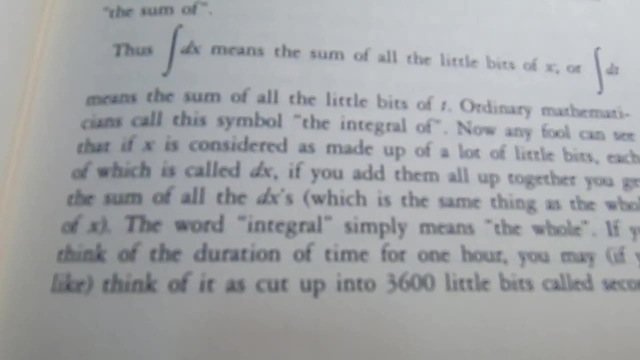 the little bits of t it says. ordinary mathematicians call the symbol the integral of like. apparently i just did. now any fool can see that if x is considered as made up of a lot of little bits, each of which is called dx, if you add them all up together, you get the sum of the dx's, which is the. 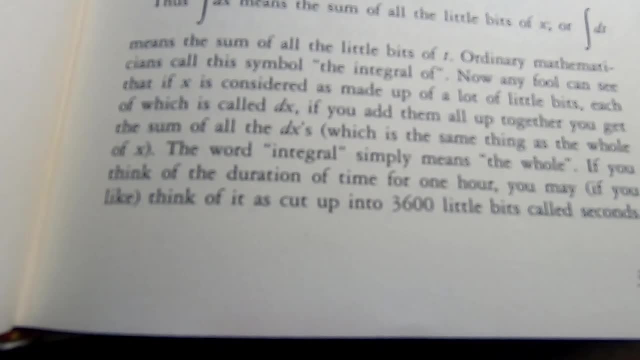 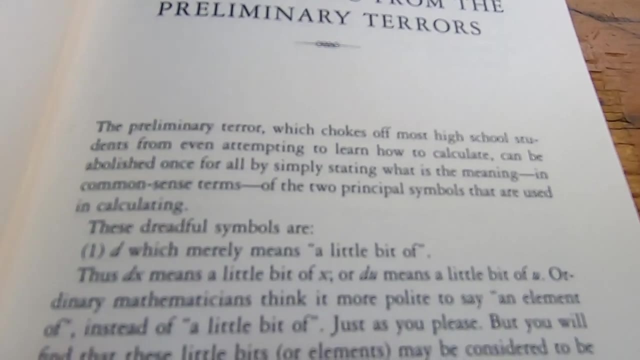 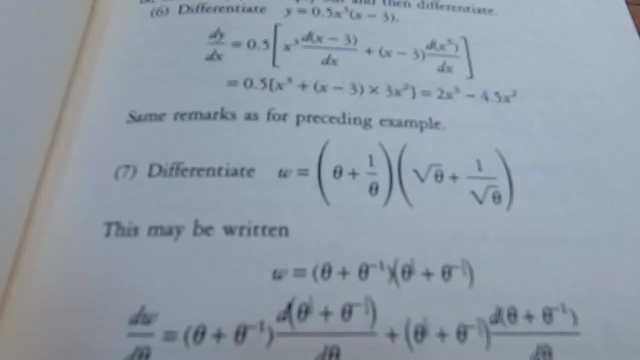 same thing as the whole of x and the word integral simply means the whole, and he goes on and gives a more concrete example. but he explains things in this way throughout the book, so it makes it a book that you can actually sit down and read, almost like a novel. so there is actual, you know, calculus. 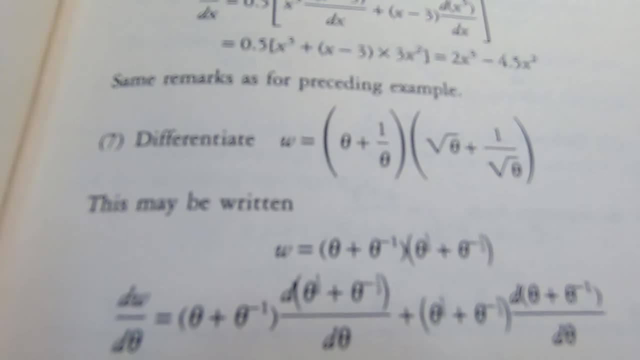 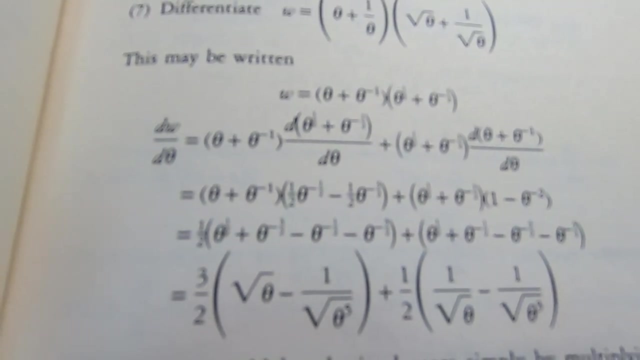 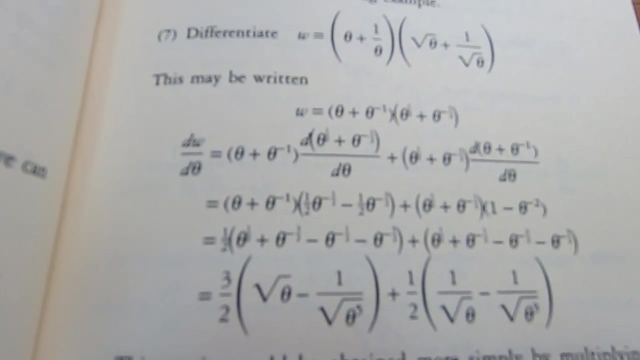 in this book there are computations. for example, here thompson finds a derivative. so you see it is a math book. it just happens to be that thompson tends to explain everything in a very elegant and well-written way, which is not common of most books. i can, i think of a handful of other books that are extremely well written. 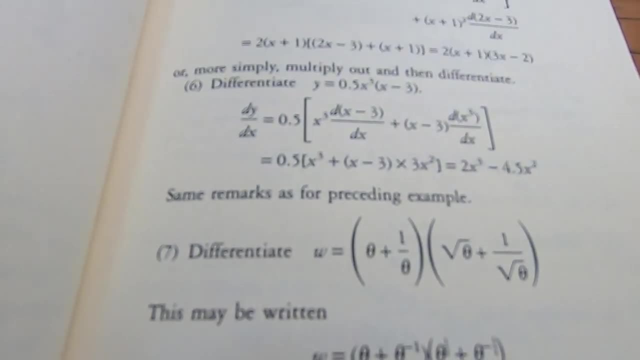 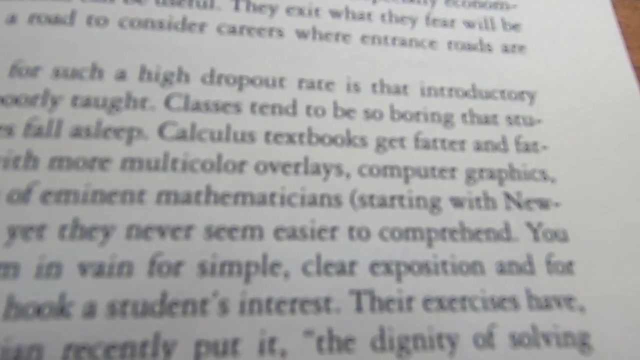 like this one, but this one is different. this one is written in a friendlier way than all of the other calculus books. i wanted to just talk about this one piece from the preface which i missed. it says: calculus textbooks get fatter and fatter every year. 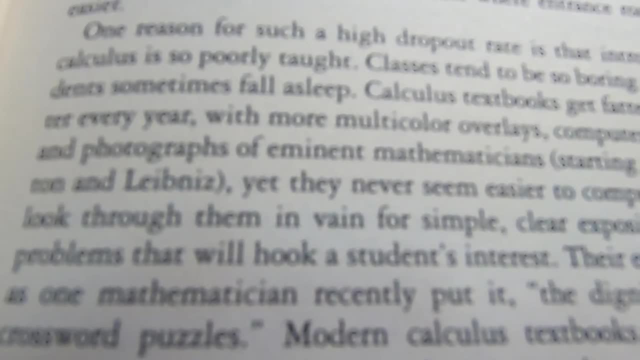 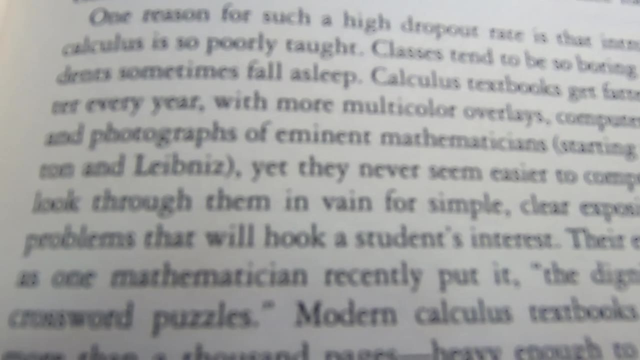 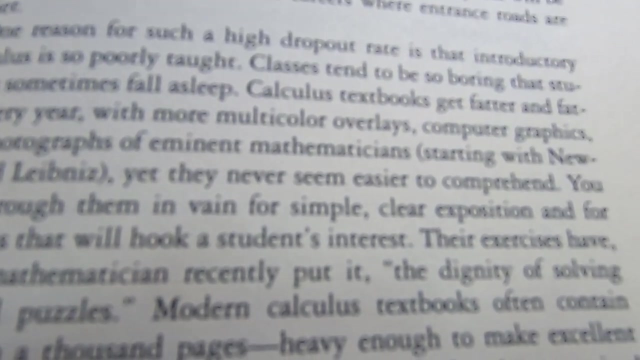 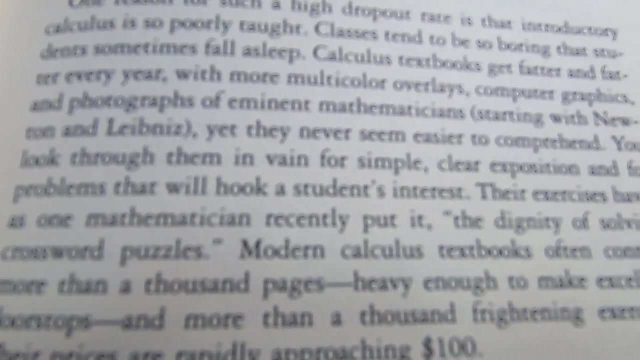 with more, more, more. their exercises have, as one mathematician recently put it, the dignity- dignity of solving crossword puzzles. modern calculus textbooks often contain more than a thousand pages. this is true, they're giant books and they have tons of examples which, which are very important to 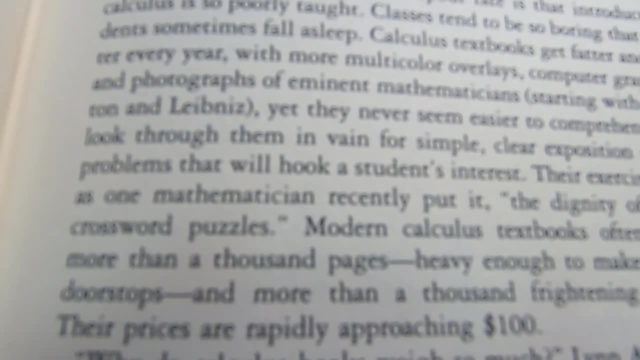 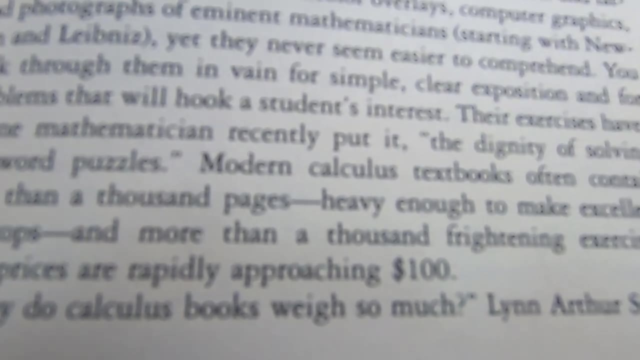 which is good, heavy enough to make an excellent, excellent doorstops and more than a thousand frightening exercises. This is true, And their prices are, it says here they're approaching a hundred dollars. So if only uh Gardner knew that they're over $300 today. Why do calculus? 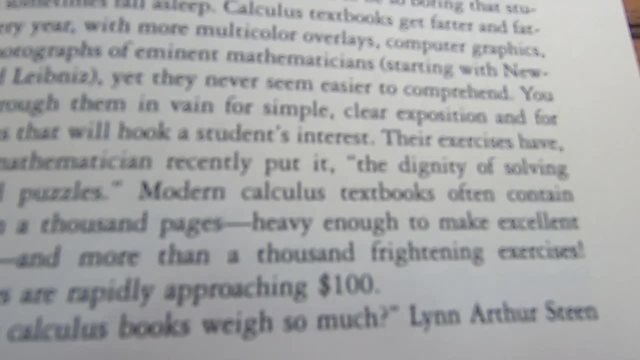 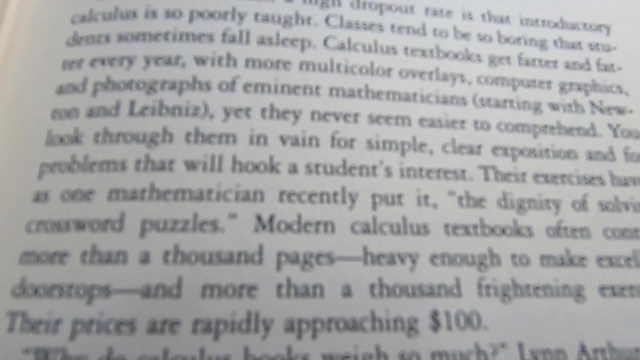 books weigh so much. Yeah, it goes on and on and on. uh, just kind of bashing the modern books. Now I do think that a big pro of the modern calculus books is that they have lots of exercises. It's really important to be able to do lots of exercises, So I don't completely agree. 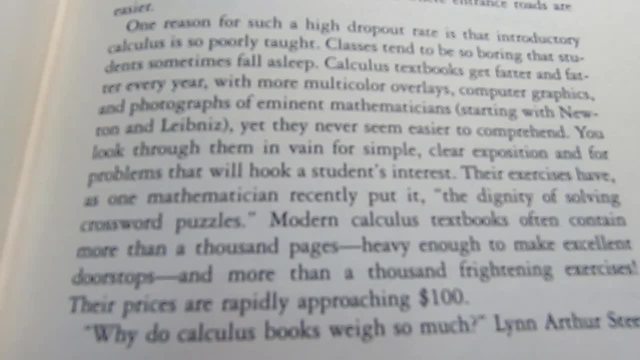 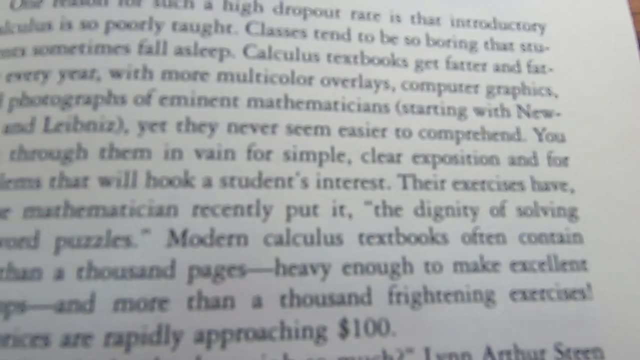 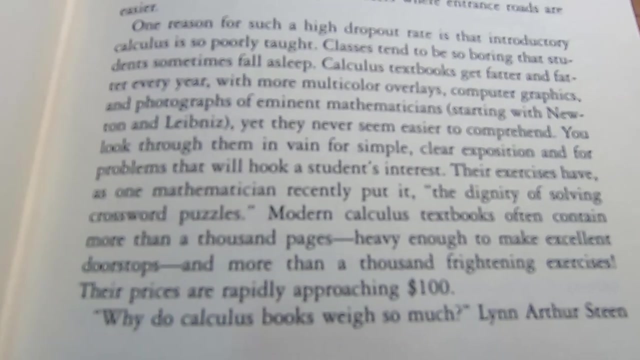 with the statement here, And while this textbook does have a lot of exercises, uh, it's definitely worth supplementing it with one of these modern ones with lots of exercises. You know I'm all about reading math, but you also have to actually work out problems to get good at math. This book 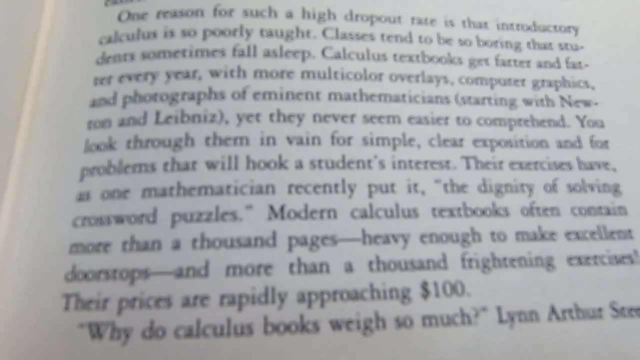 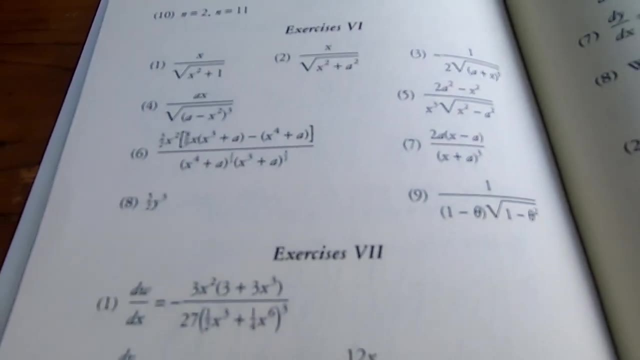 does a really good job with the reading. I think this is the back of the book, So you do the. Okay, I'll just do the bottom and then the top part of it. Okay, So you do the coordinate analysis. you see that the author did include exercises, which makes it really really good for self-study. 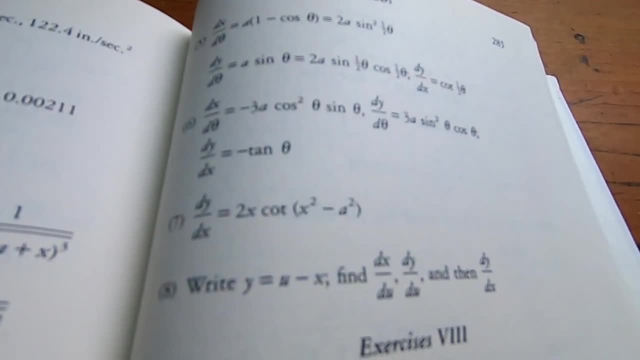 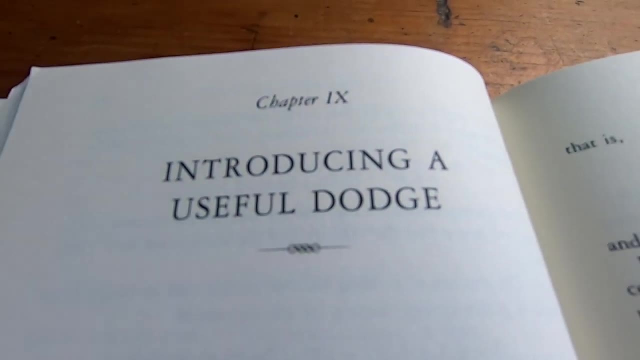 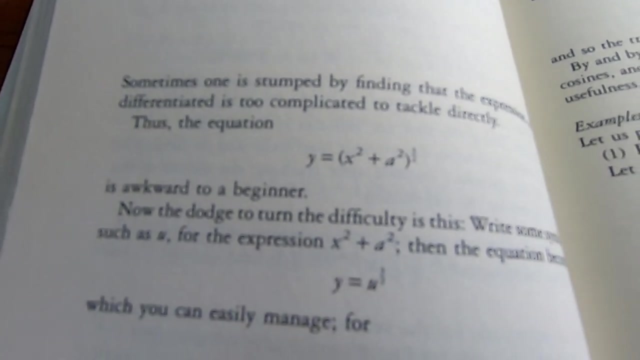 So very, very, very, very useful. This is a chapter in the book. He calls it Introducing a Useful Dodge- I love the language of Thompson- And basically it's just a substitution. He introduces a method of substitution which makes things easier for some people. I personally don't use this method. 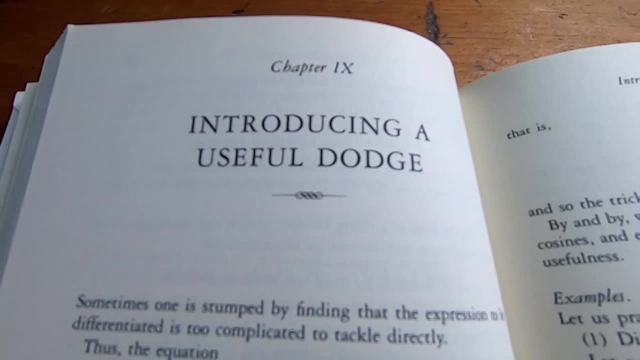 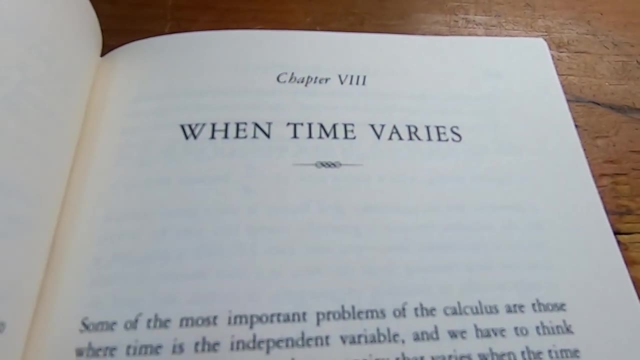 But I could see its value right, I can see the value in it And I appreciate that he has a whole chapter on it, So I think that's kind of good, One of the big pros of this book, and I think I 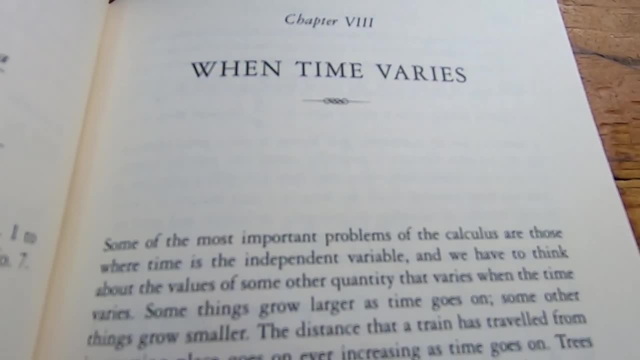 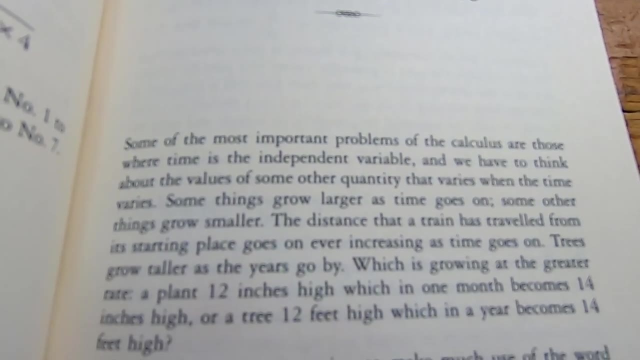 already mentioned it is that you can kind of just like lay in bed and read it before you go to bed at night. It reads really really well And you can read it and understand a lot of it without having to write anything down. Obviously, how much you have to write down will depend on how 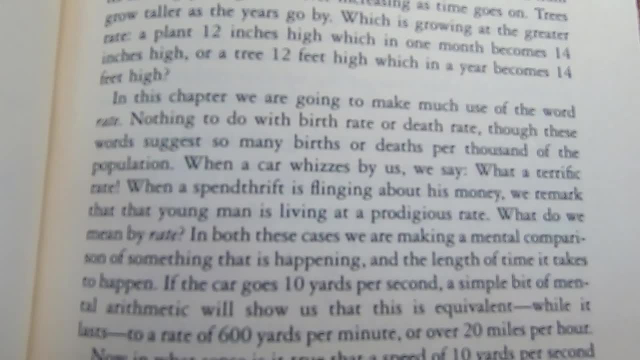 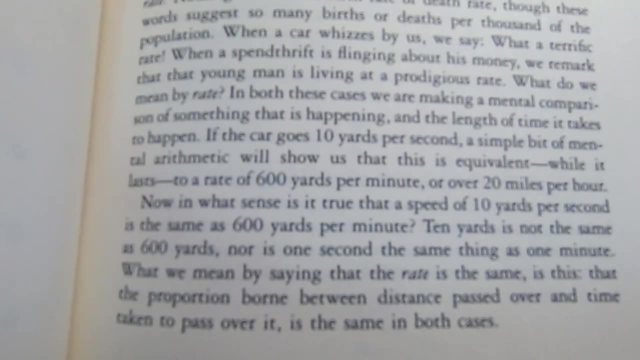 much calculus, you know. But look, there's no math on this page. It's just explanations in words And there's numbers, And so there is some math. But it's stuff you can do in your head because he's explaining it for you, So you don't really need 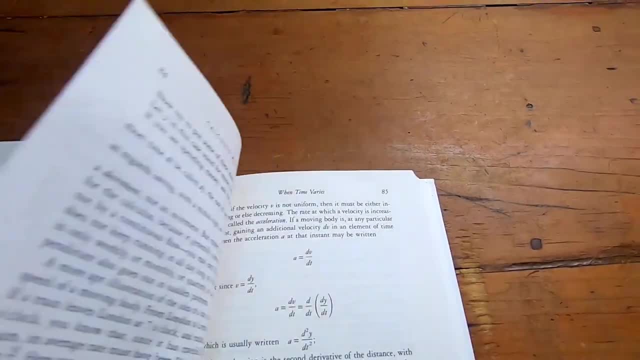 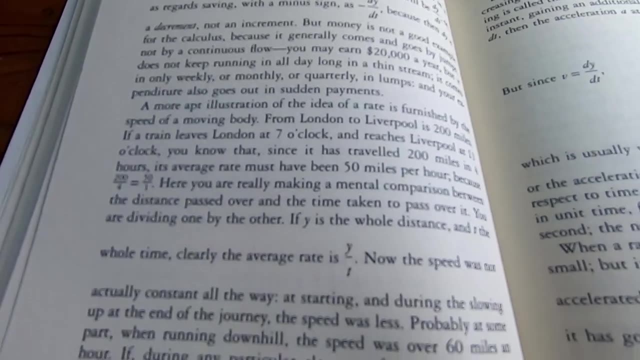 to have a piece of paper to read this entire page. Let me turn the page and show you And see here he keeps going. He's just explaining stuff right, And so you can kind of read it like a novel And you get a lot from that. You get a lot from reading, you know, I know a lot of people. 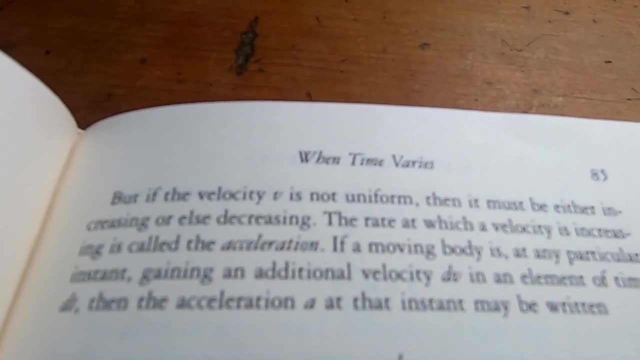 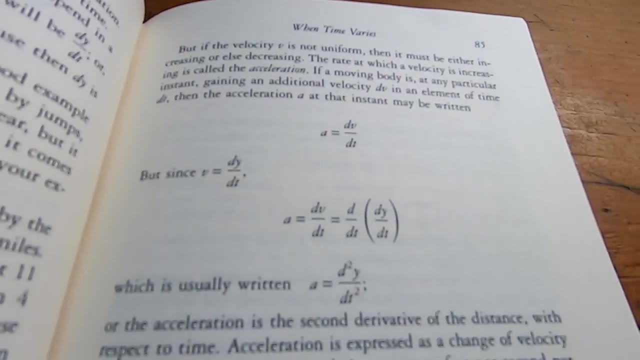 are a big fan of videos, And I'm one too. I mean, I make YouTube videos, But I don't know if you've read any of his books. I don't know if you've read any of his books, But I'm an even bigger fan of reading. I feel like I learn more from reading books than I do from. 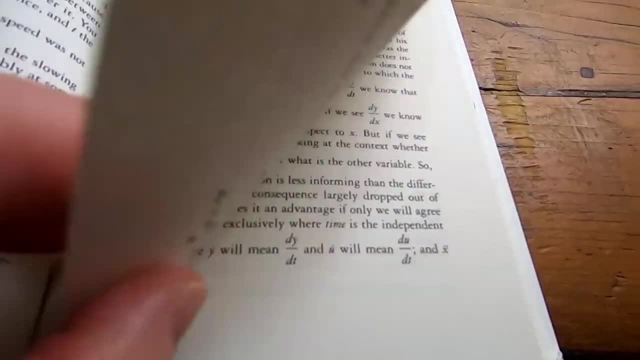 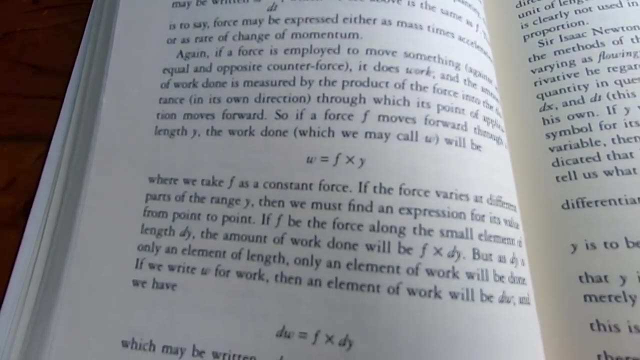 watching videos. Let's just keep going with this chapter just to show you. Look, it's just more and more words And he just keeps explaining and explaining. So you could keep reading all of this and probably understand all of it without writing anything down. So it makes it kind of. 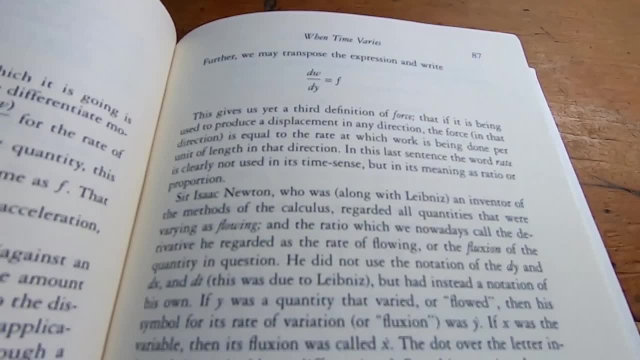 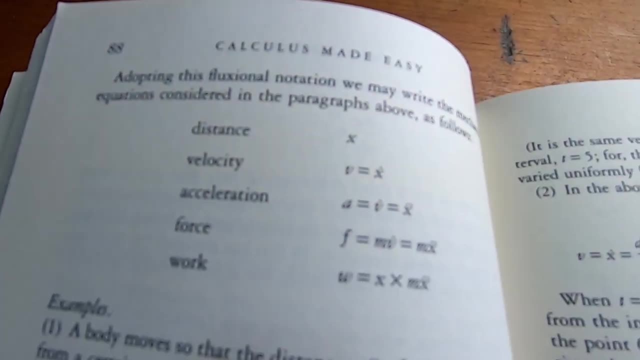 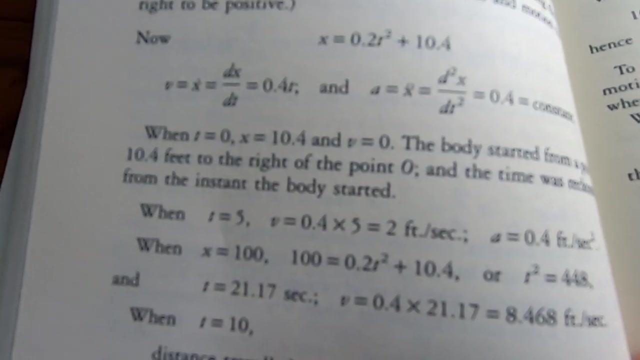 like a casual reading calculus book, which is not something you find in modern textbooks, right? I mean, look, all of this is still casual reading in a sense. Now, here there's some computations, right? So if you wanted to verify these, you would have to do. you know some math, But it's still. 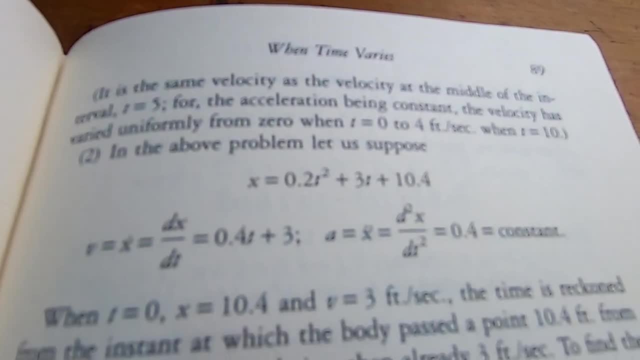 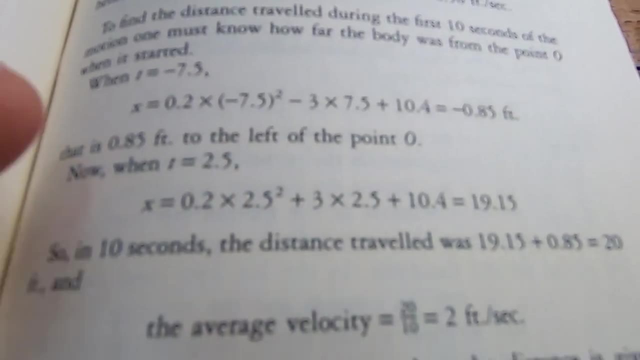 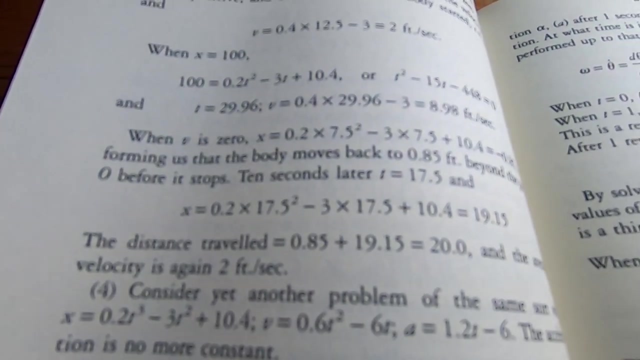 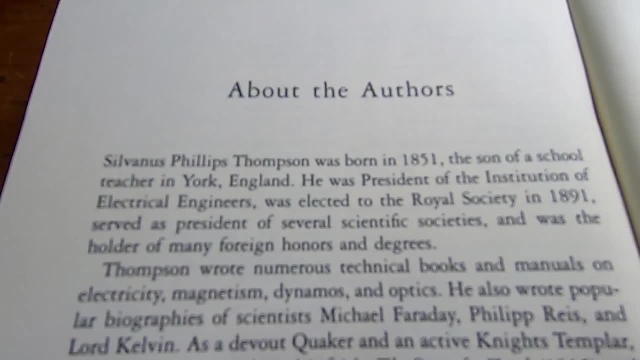 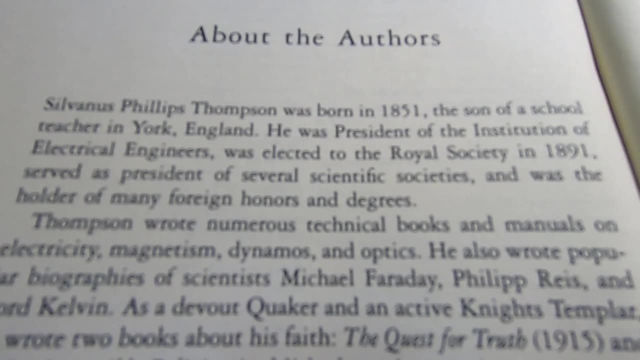 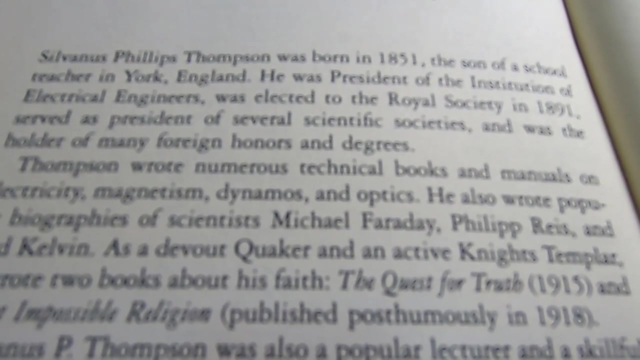 Thompson, which I looked up on Wikipedia, by the way, before making this video. The guy was legendary. It says Thompson was born in 1851, the son of a school teacher in York, England. He was president of the Institution of Electrical Engineers, was elected to the Royal Society in 1891, etc. etc. 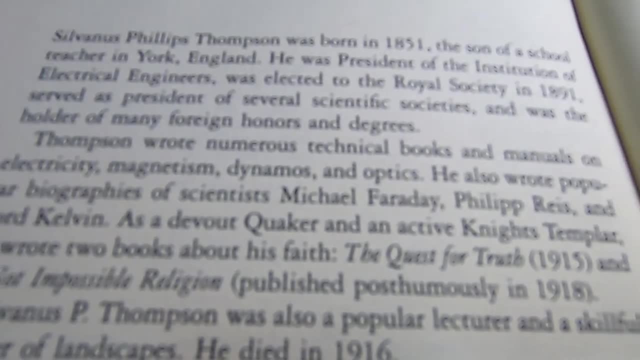 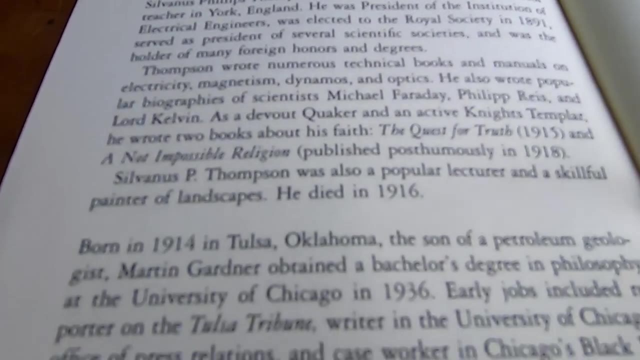 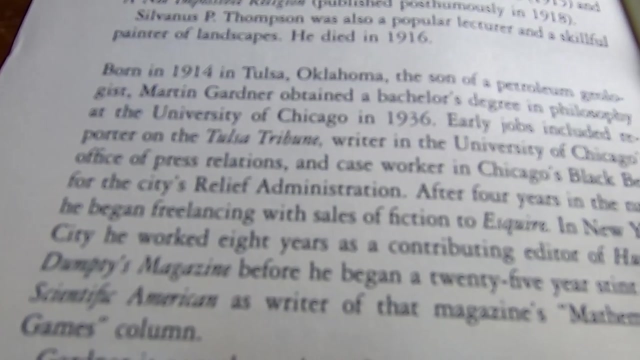 etc. So he had holder of many foreign honors and degrees. The guy was a genius, So really really impressive. Here it talks about Gardner. born in 1914 in Tulsa, Oklahoma. the son of a petroleum geologist, Gardner obtained a 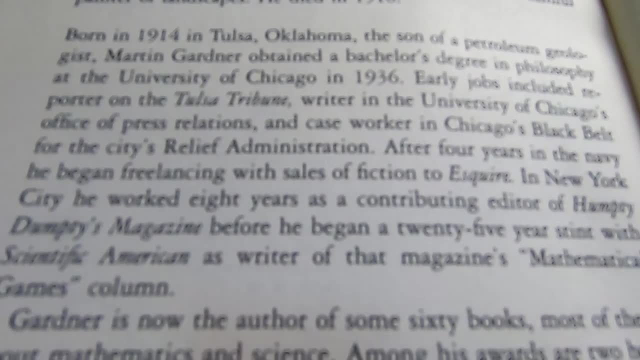 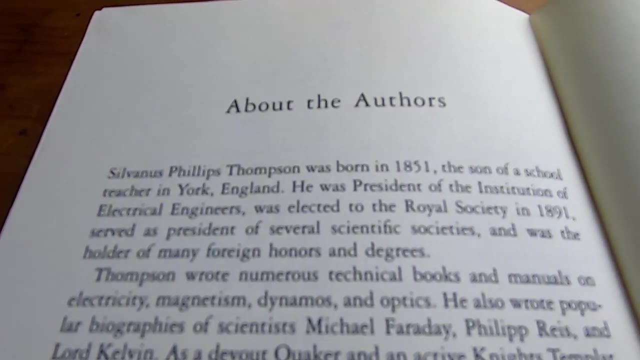 bachelor's degree in philosophy at the University of Chicago in 1936, etc. So it's really nice to hear you know about the people who wrote this book, Because when you read a book that's this good, you wonder like, wow, who wrote this And why is it not being used at more schools in the 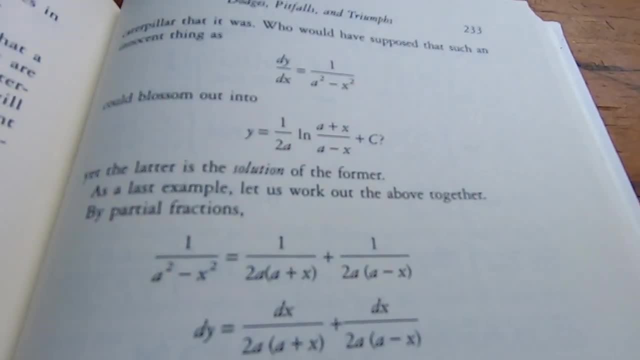 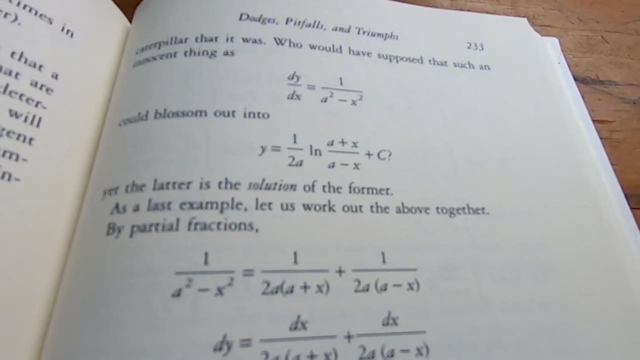 world. This is just an amazing book. So while I do think this is an amazing book- and again, I think it's probably one of the best calculus books, if not the best calculus book for beginners- It's a must read for anyone, for anyone who does math- There is a downside to this book, And that I think. 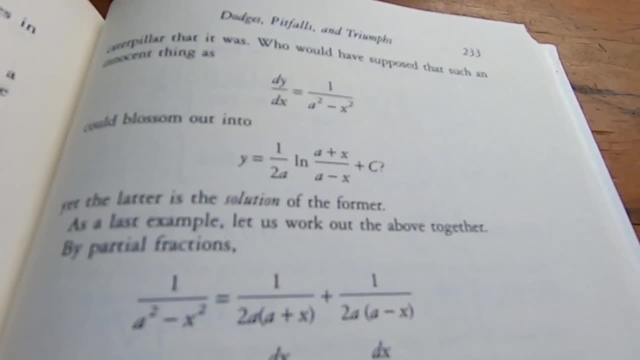 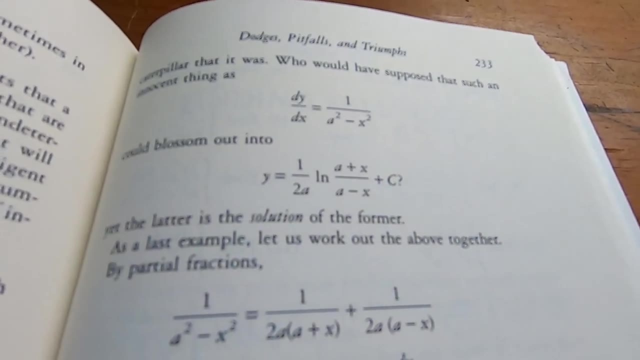 is the number of exercises. Now I know in the preface it mentions that you know the modern books have, you know, thousands of problems and kind of put that as a negative. I do think it's important to do lots of exercises. So I do think if you're genuinely trying to learn calculus and 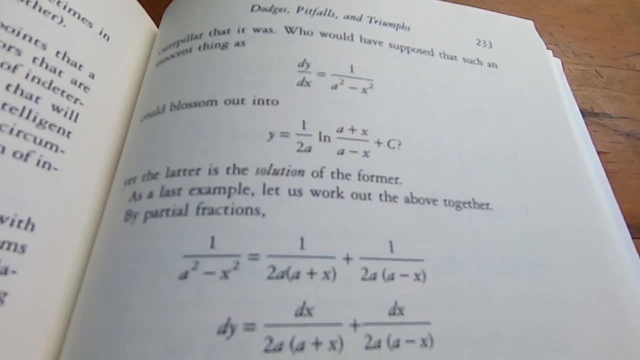 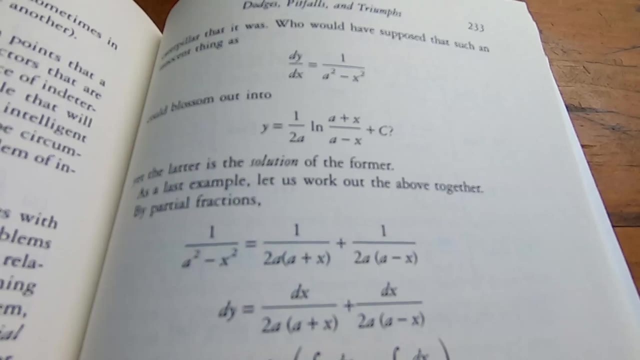 you're using this book, you should also pick up, you know, one of those modern books that's that you can use as a doorstop And you don't necessarily have to read it. but you should do the exercises right. They provide lots of practice problems which are useful to do when you're. 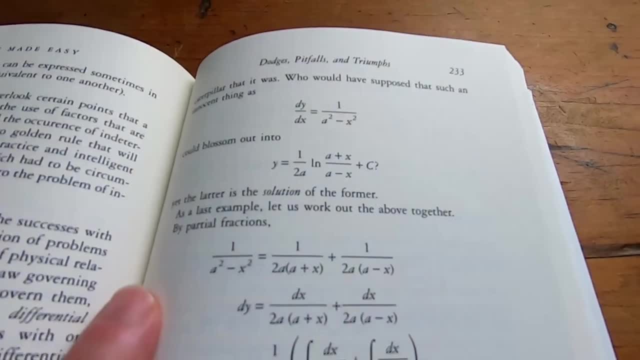 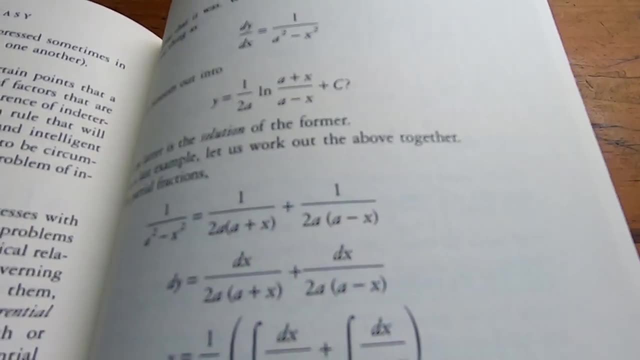 learning a new subject. So I would say, for anyone wanting to learn calculus, get this book and then pick up another book, like you know, one of the more modern ones, like the book by Stuart or the book by Larson, and just do the exercises out of those and read this one. right, Cherish this one.